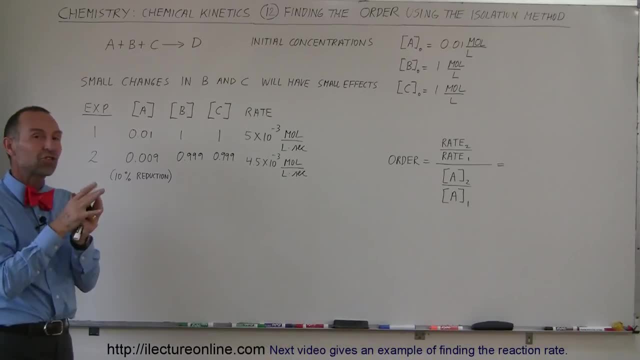 such a way that when it gets used up during the reaction, the change in the concentration is negligible compared to the concentration of the one that we're really interested in. So we want to know what the order is for A, and we want to somehow make B and C. 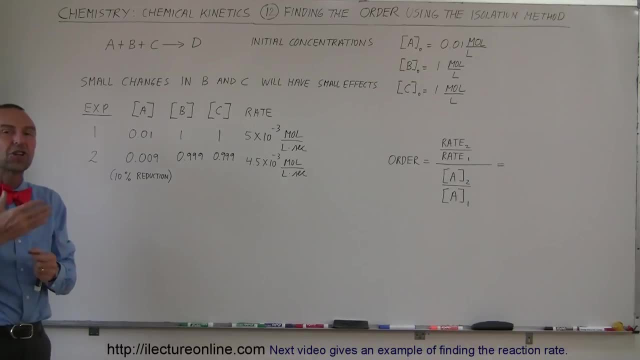 non-players in the reaction. Non-players meaning that the change in their concentration is, relatively speaking, very small, so there's no effect on the reaction. So small changes in B and C will have small effects. that's what we're after and the way we do. 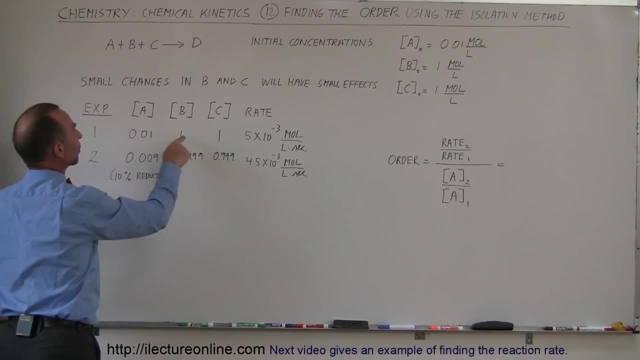 that is, to have the concentration of A to be relatively small compared to the concentrations of B and C. So this is in moles per liter. so the molarity here would be 0.01 versus 1 and 1 for B and C. At that point we find that the rate is equal to 5 times 10, to the minus 3 moles per. 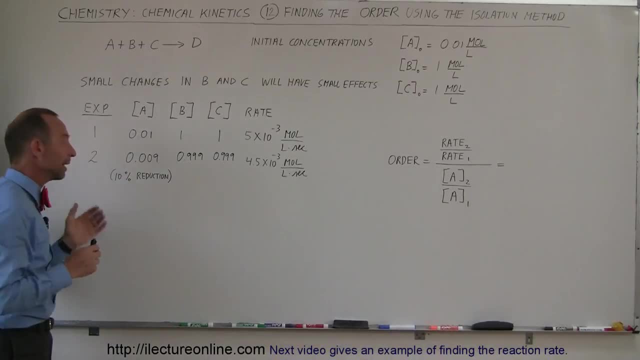 liter per second. Now we're only going to change- well, actually we're changing- the concentration of all three, but only this has a large effect. For example, when we change it from 0.01 to 0.009, even though in molar terms it's very small. 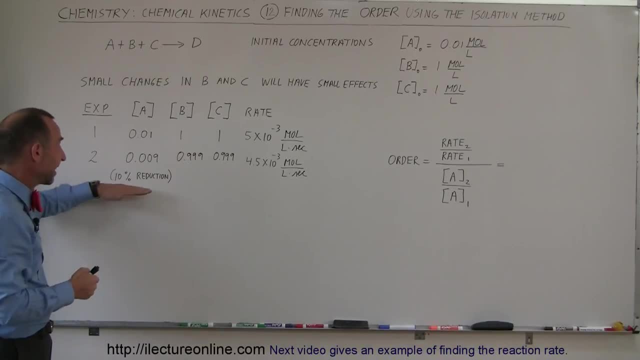 going from 0.01 to 0.0009. that's a 10 percent reduction in the concentration, Although for B and C that's only 0.1 percent reduction in concentration, in such a way that this will have very, very little effect on the rate of the reaction, where this will have the 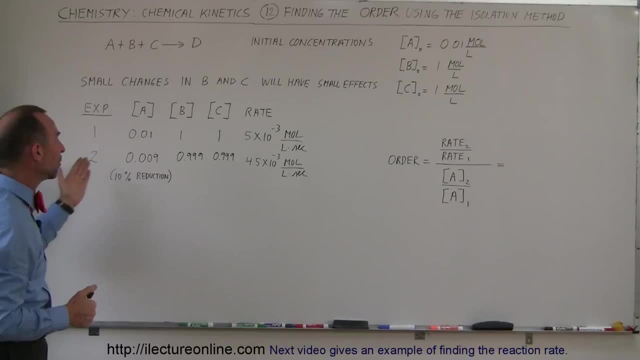 vast majority of the change in the reaction. And then if we measure the reaction rate, we can see that it's now for: instead of 5 times 10 to the minus 3, it's now 4.5 times 10 to the minus 3. 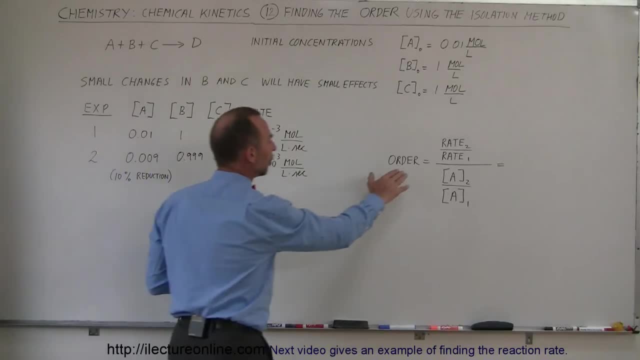 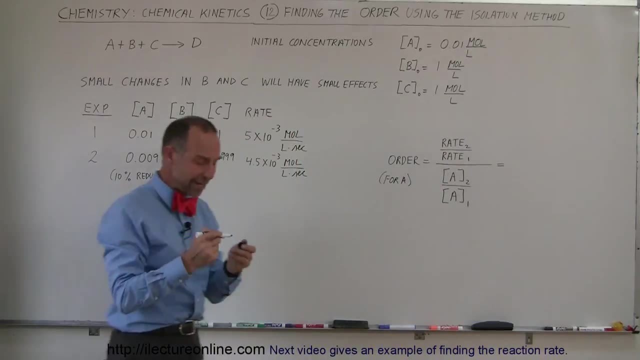 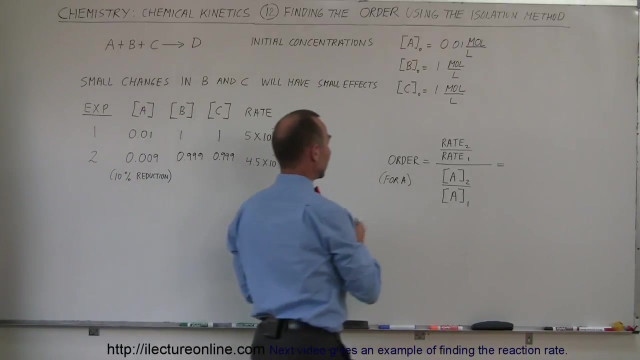 moles per liter per second. So if we're trying to find the order for A, of course this is of course. for A we take the ratio of the rates when we have a lower concentration, A compared to when we have a higher concentration of A. So in case of this example right here, that means we're going to take 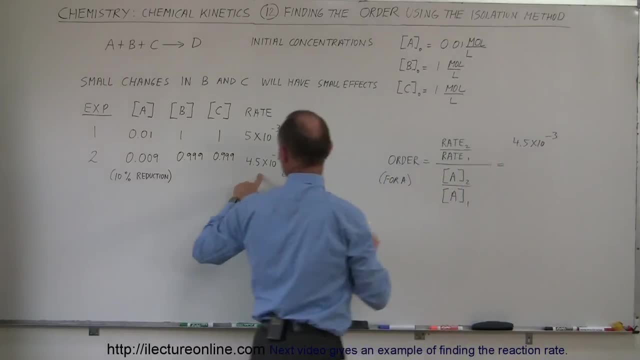 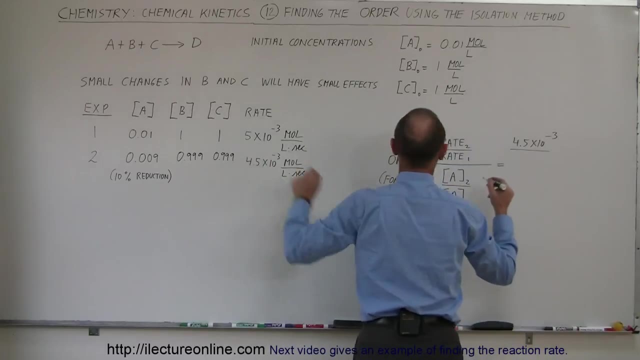 4.5 times 10 to the minus 3, which is the rate, the second experiment or after we've exhausted 10 percent of the concentration of A, and we divide that by the initial rate that we started with at 5 times 10 to the minus 3, and we divide. 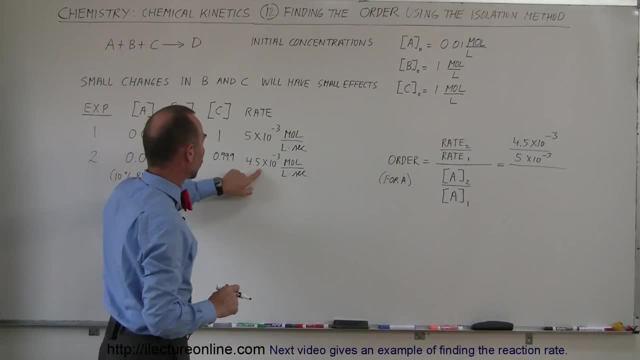 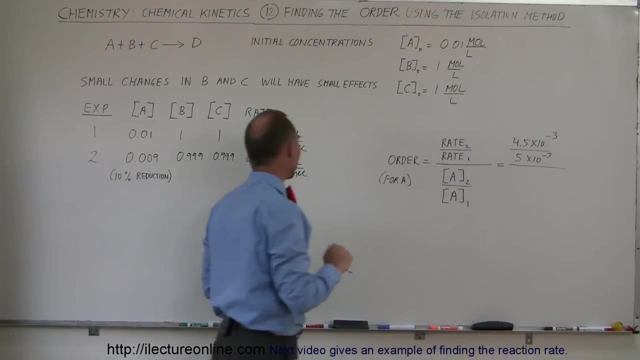 that by the change or the ratio of the reaction rates. So the second reaction rate is 4.5. oh, wait a minute. oh, we have the rate. I'm sorry, I'm going for concentration. I was going to do the rate twice, but no, what I want to do now is the ratio of the concentration, so it's 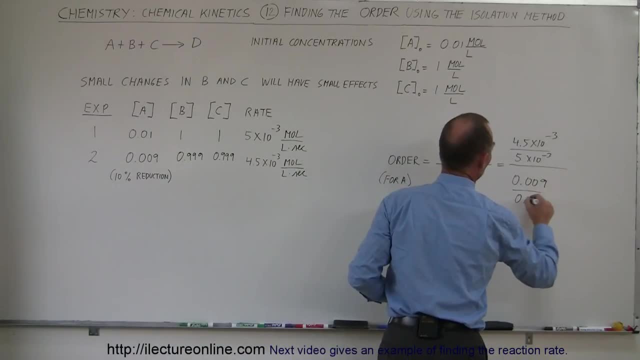 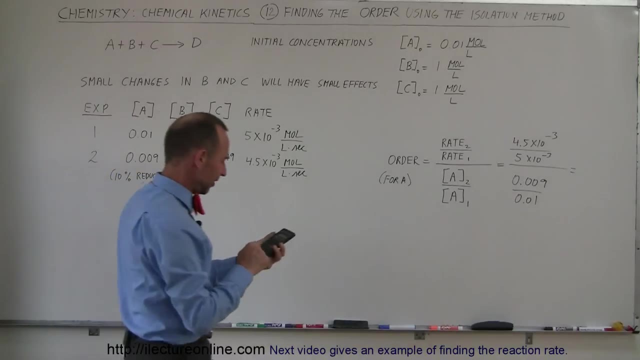 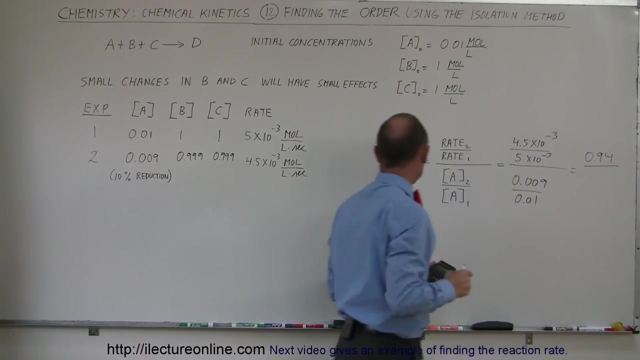 0.009 divided by 0.01. and let's see what that gives us. so if we divide 4.5 by 5, 4.5 divided by 5 equals that gives me. that gives me 0.94, 0.94. and we divide that by the ratios of the concentration, that would be 0.009 divided by. 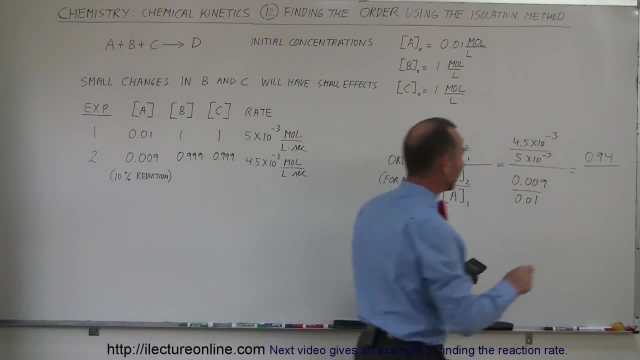 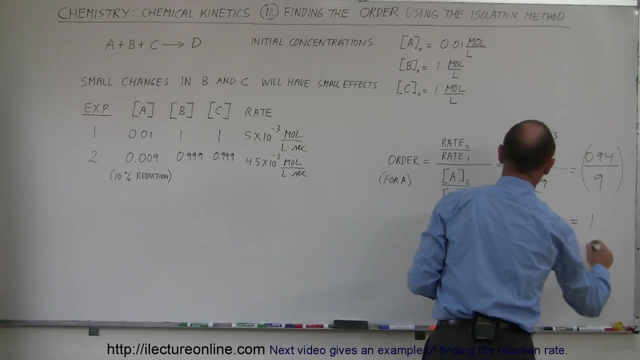 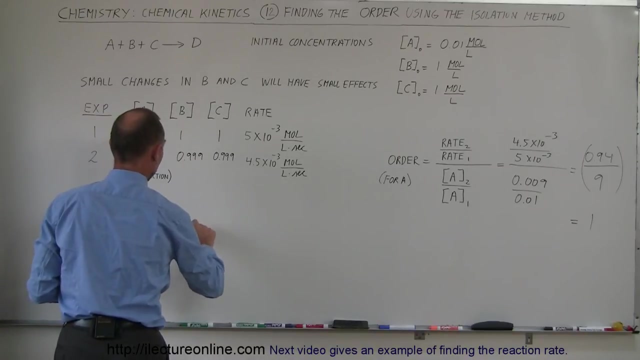 0.01. I don't really have a media calculator for that. that is equal to nine, but you can see that that is roughly a one-to-one relationship. so this is roughly one. that means that the order of A is one, and if we then write the equation, we could then say that the rate is equal to the reaction. 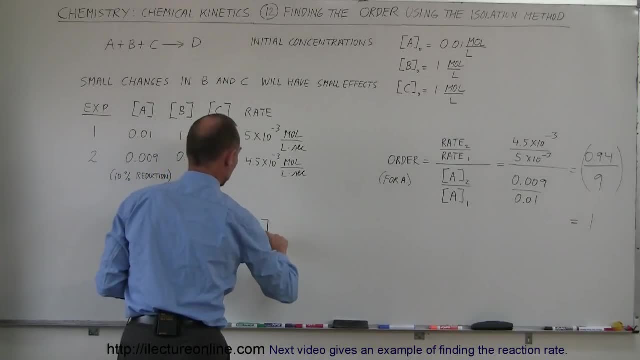 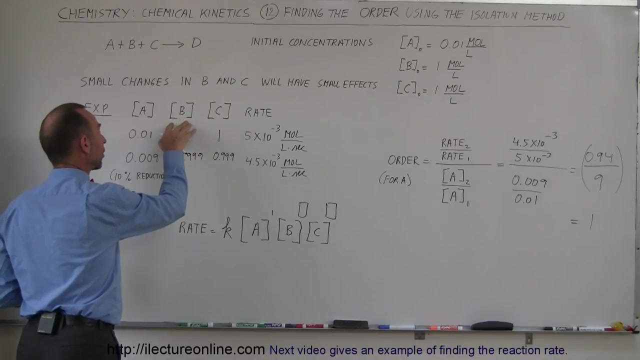 constant k times, the concentration of A to the first power, the concentration of B and the concentration of C. Well, that we don't know yet. Well, we then would have to do this experiment again, but in this case, the second time, we would keep plenty of concentration of A and then reduce concentration of B to a very small. 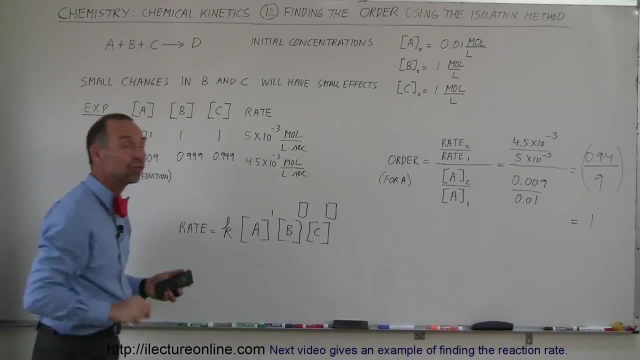 amount, then reduce it maybe by 10 and see how the reaction rate changes then. and then we find the order of B, and then again we do the same thing, but now we make A and B very concentrated and C just with a small amount of concentration there, and again we allow C to change, and then we find the order for C, and that's how we go ahead and do that, and that's what we call finding the expansive reaction after A and C, Counting concentration B by producing less until certain fryhta to C and then reducing it by 2 to C, and so forth.